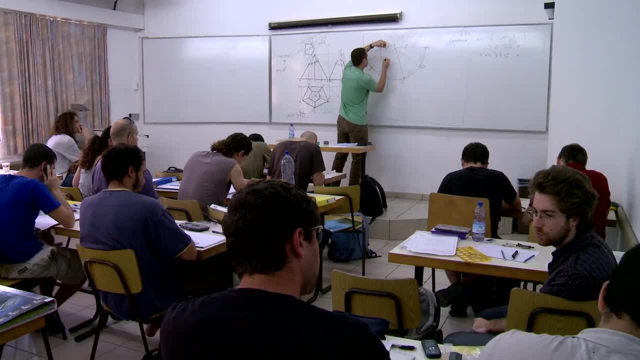 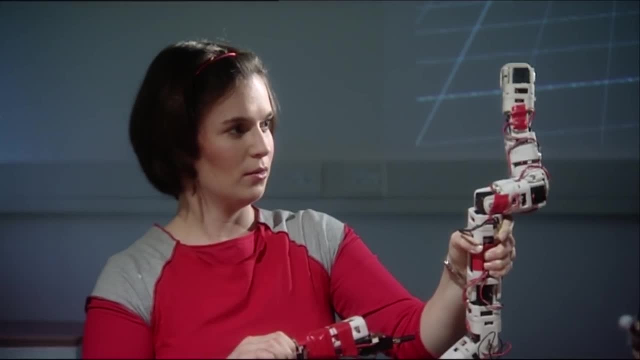 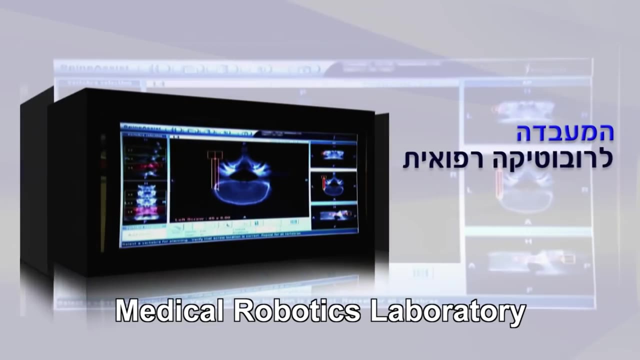 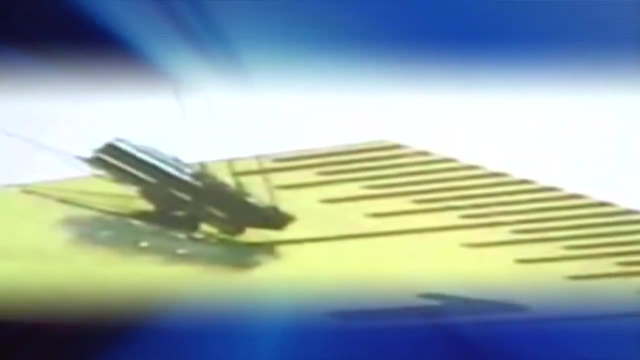 of engineering and the major sciences. Major tracks of study in mechanical engineering include dynamics, mechatronics, robotics, mechanics and biomechanics, energy and flows, CAD manufacturing and control. Professor Moshe Shoam, head of the Medical Robotics Laboratory, has developed a miniature remote-controlled 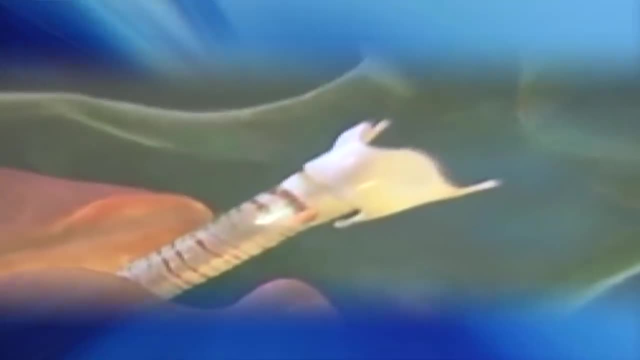 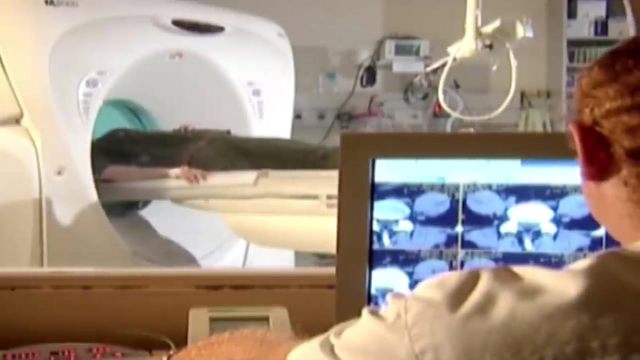 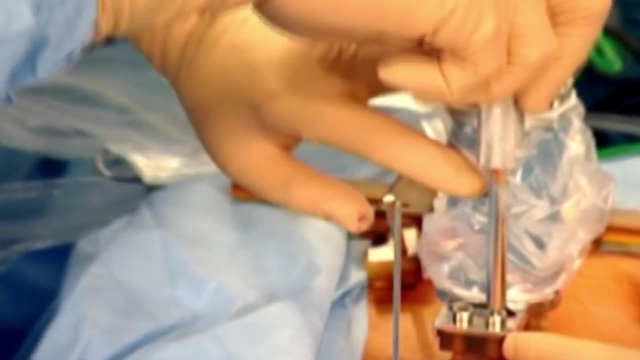 robot that can move independently through the body's channels, veins and arteries, thus facilitating diagnosis and medical treatment without human intervention. Another application developed by Professor Shoam, already in use today, is a miniature robot that performs complicated surgeries on the spinal column with greater precision. 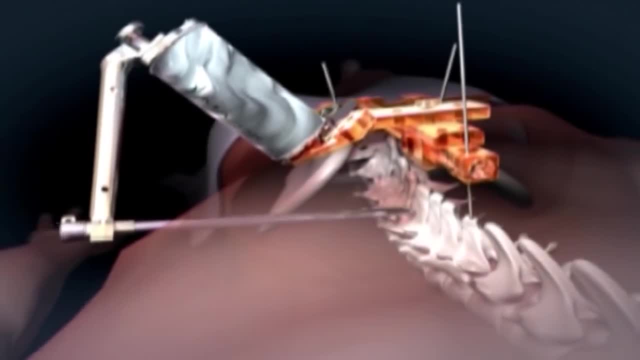 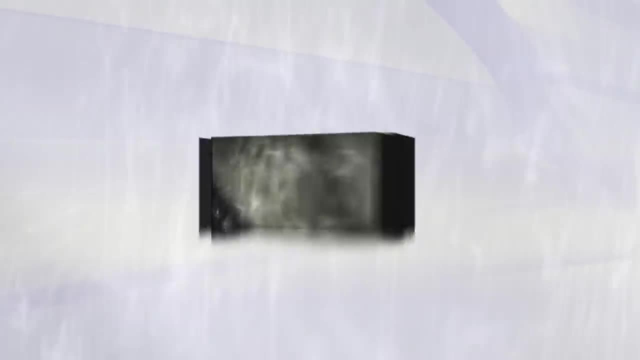 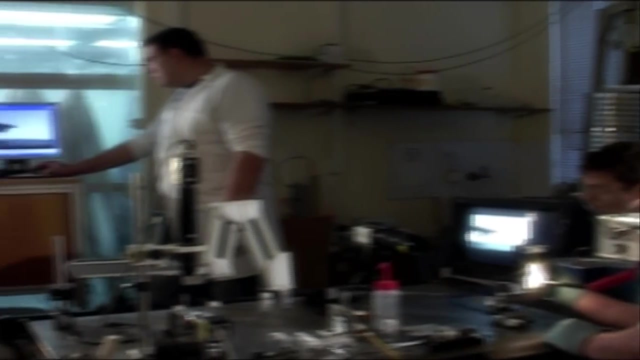 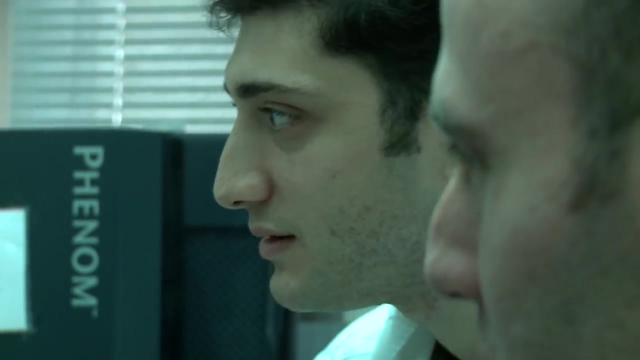 than that of a surgeon. This development is already saving lives around the world. Here in Professor Eyal Zussman's lab, Professor Shoam is working on a new robot which is designed to be able to move around the body's channels, veins and arteries. 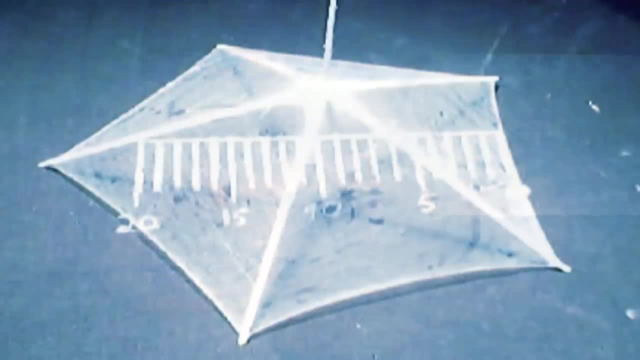 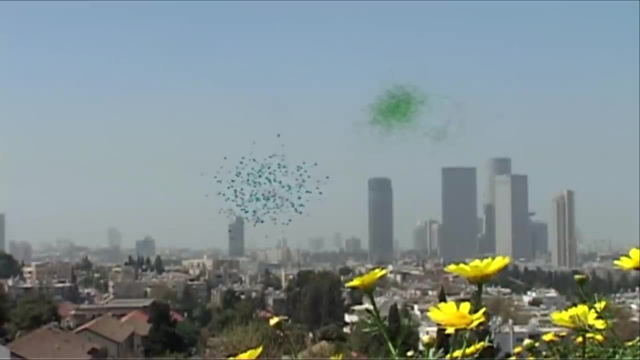 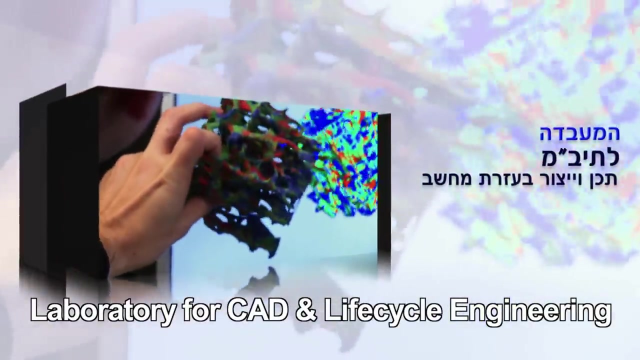 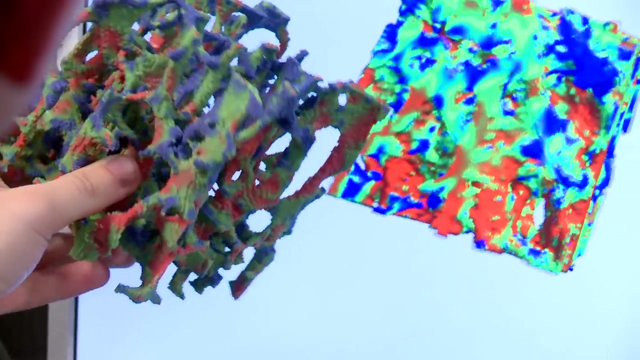 The robot is designed to be able to move around the body's channels with greater precision than that of a surgeon. The robot is designed to be able to move around the body's channels with greater precision than that of a surgeon. Until recently, the word teleportation was mainly know only to science fiction writers. 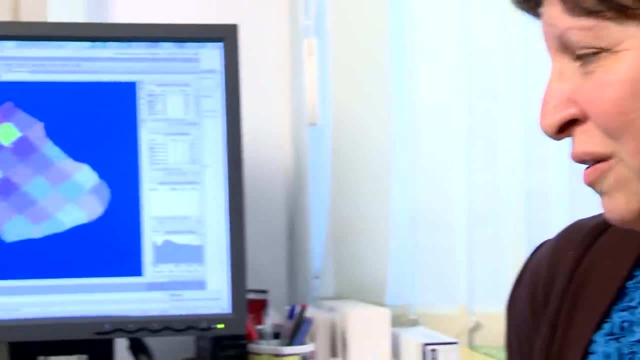 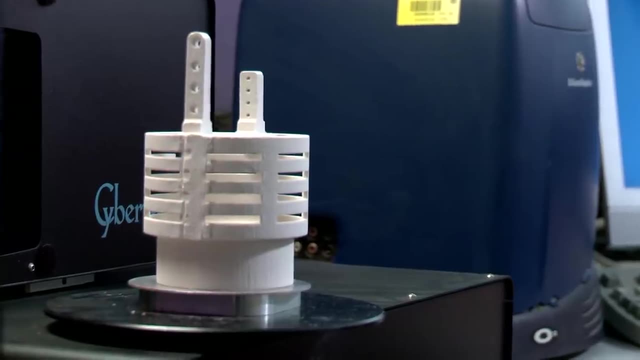 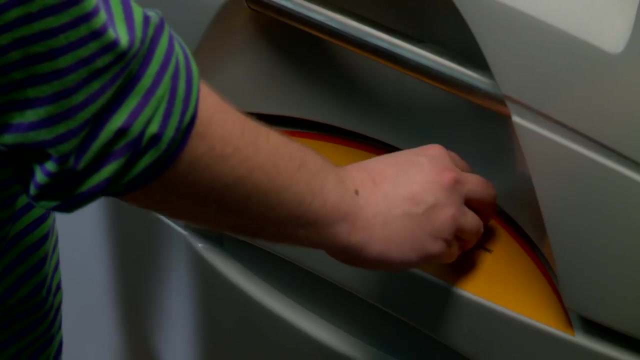 Today, Professor Anat Fisher and her CAD Lab research team are developing advanced methods for modeling, simulation and analysis based on engineering and medical CAD systems. One of these systems- This system- enables scanning a three-dimensional object and creating a model which then serves as a basis for design, computerized analysis or manufacture by digitally transporting the model to a three-dimensional printer. 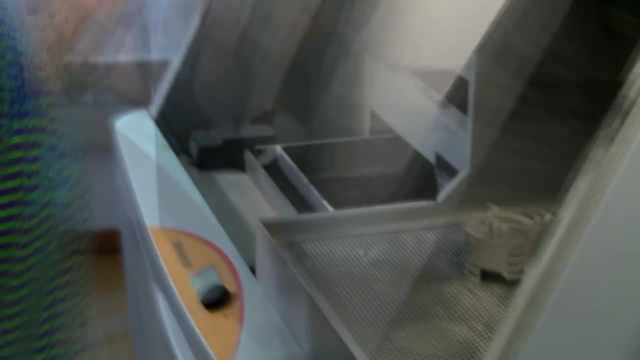 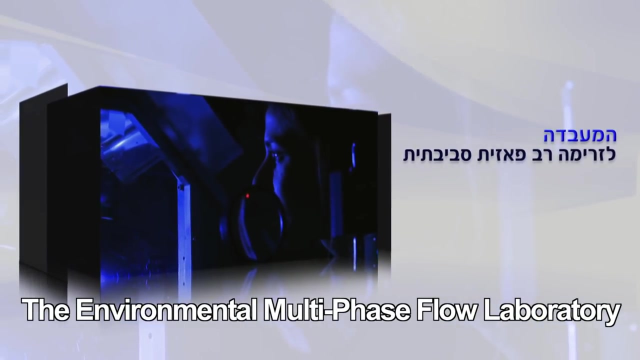 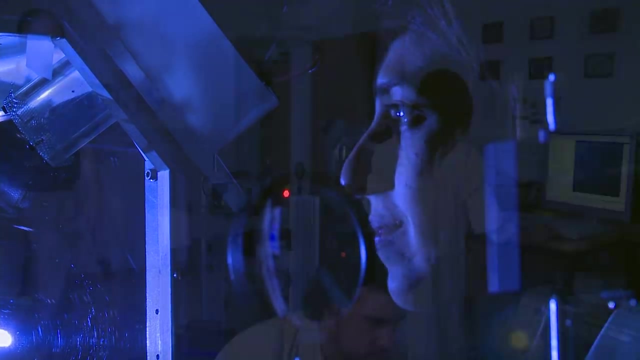 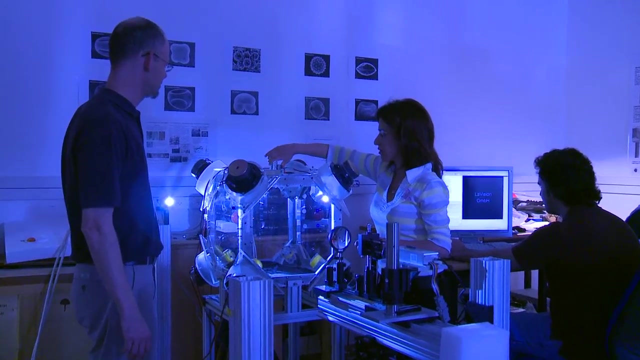 Dr van Hout. investigates multi-phased flows, in particular, to examine environmental problems caused by bioaerosols and particle behavior in a turbulent flow. These phenomena play an important role in industrial and natural processes such as erosion. Understand the role of bioaerosols in the development of natural processes. 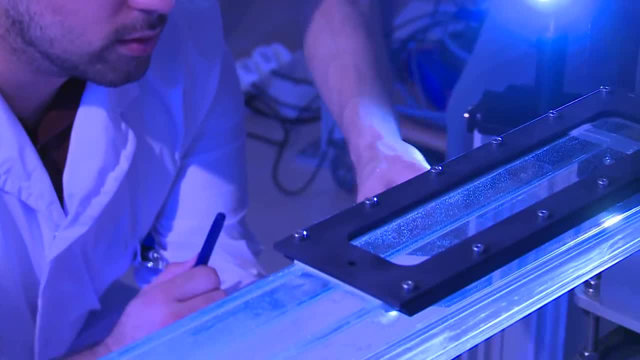 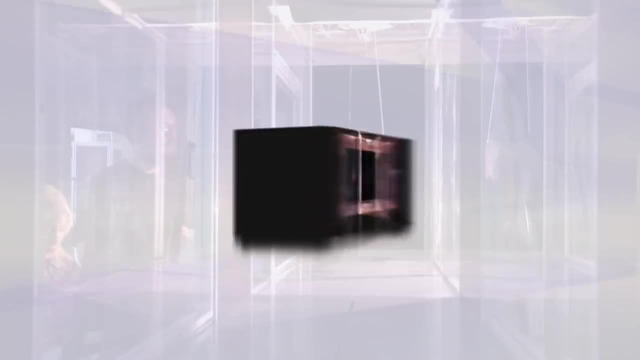 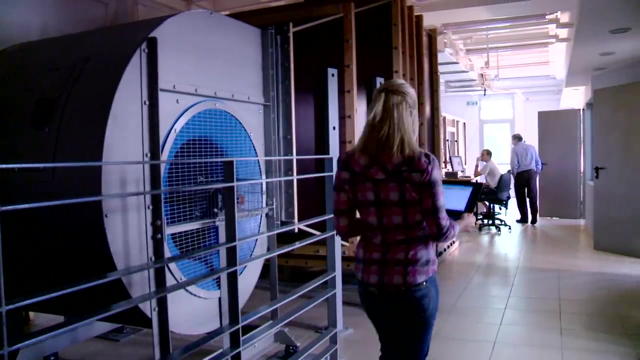 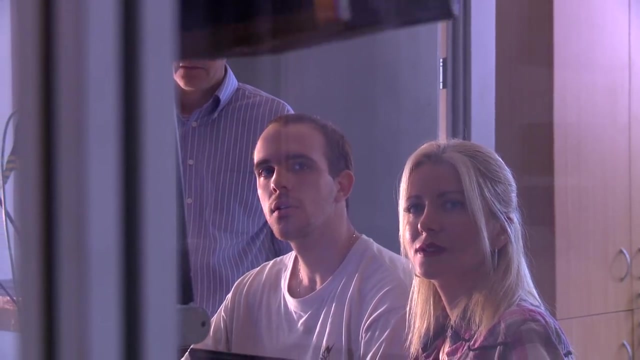 Understand the role of bioaerosols in the development of natural processes. Understanding how related bodies interact with the flow surrounding them is an important factor in chemical engineering. Research in Dr David Greenblatt's lab focuses on creating models to demonstrate how objects react under the flow of energy in a wind tunnel and a water tunnel. 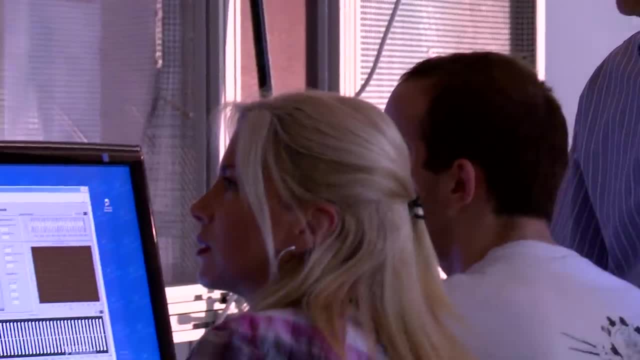 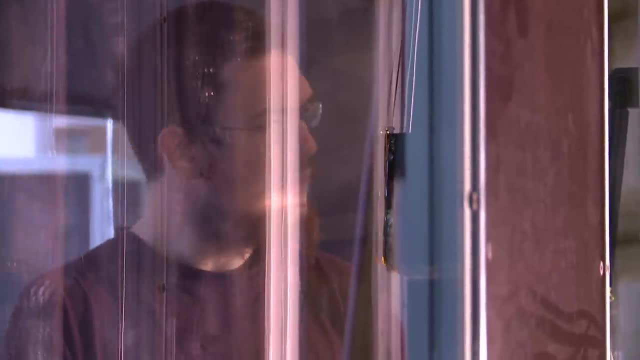 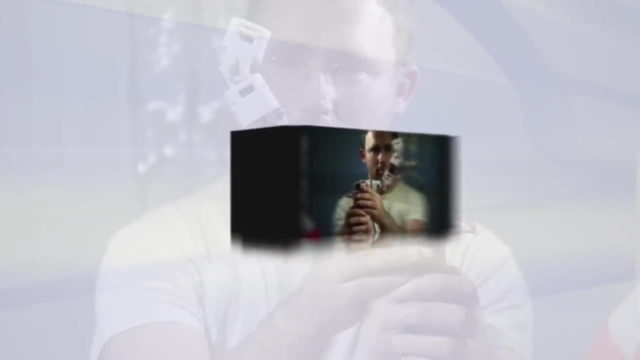 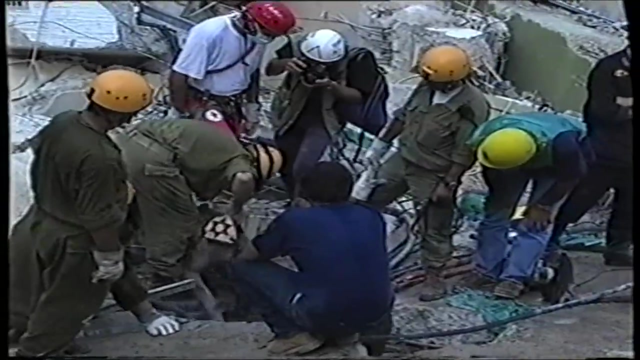 The flow of energy is controlled in numerous ways, Among them electromechanics, voice wave control and plasma. This research is intended to improve the energy efficiency of equipment such as fans, pumps and computer cooling systems. Humans have always found inspiration for solving their problems in nature. 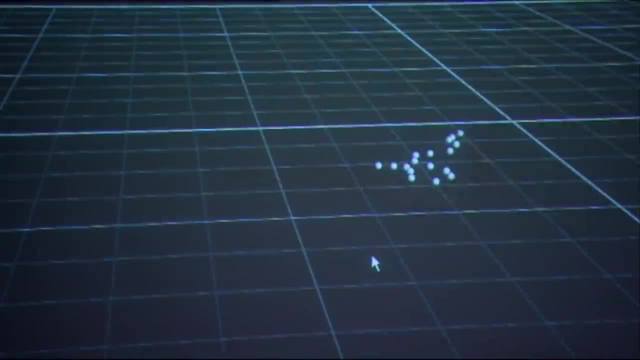 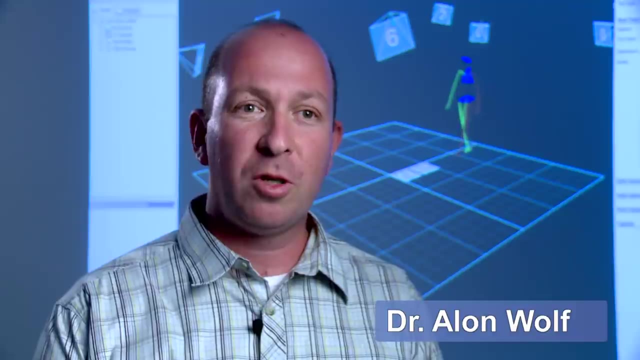 The same applies to Dr Alon Wolf's lab, where researchers have studied the effects of bioaerosols on humans. We study and investigate how snakes move. We observe and monitor how animals move, particularly the kinetics of this motion. We observe and monitor how animals move, particularly the kinetics of this motion. 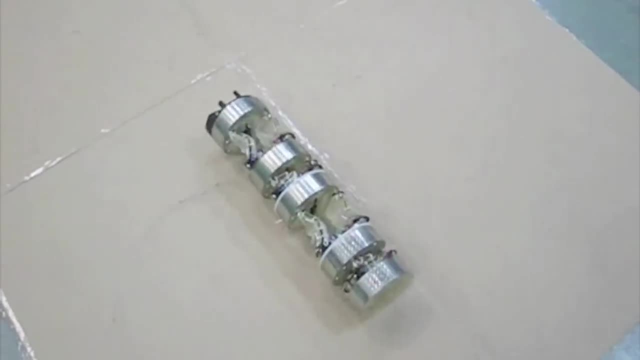 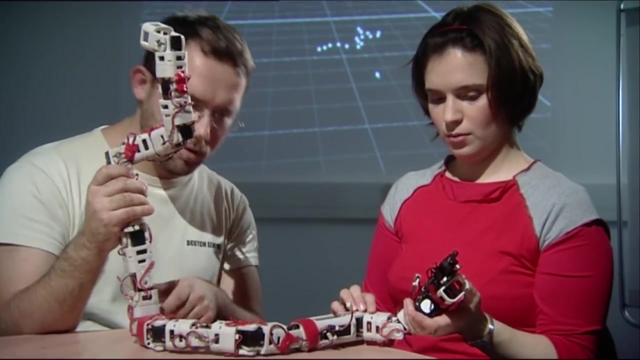 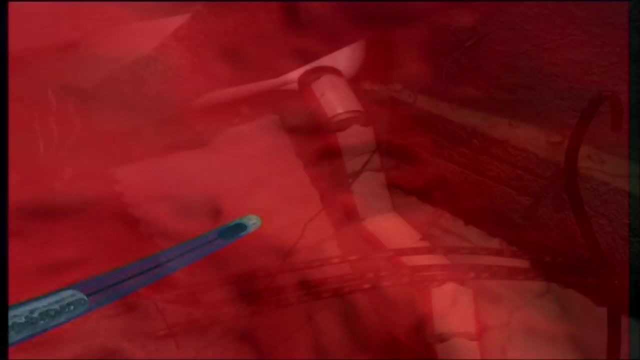 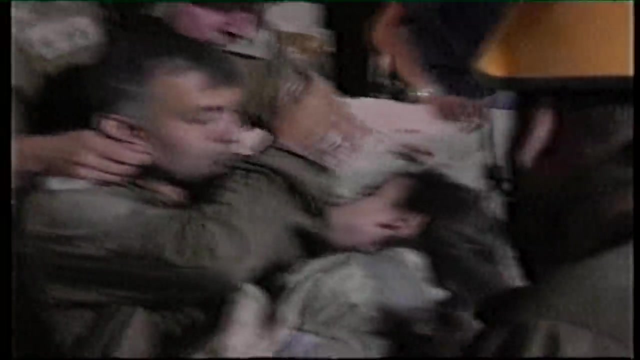 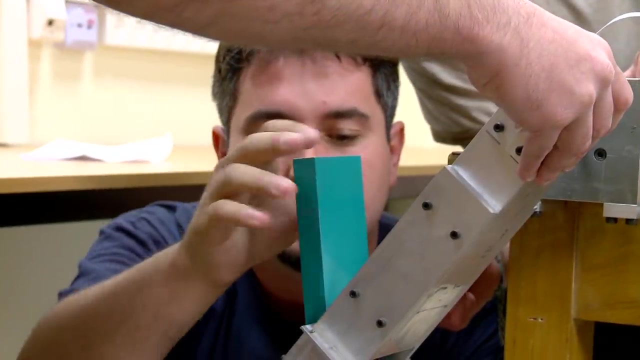 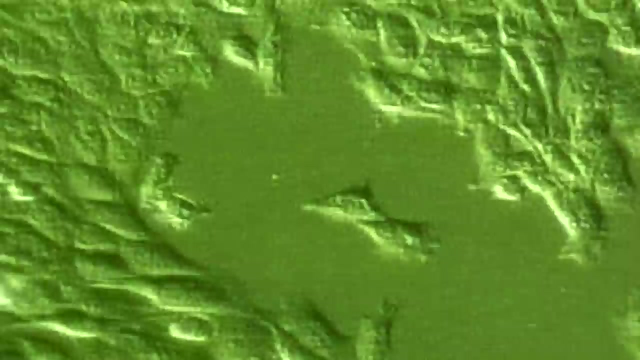 We then attempt to adapt these behaviors into robotic systems, producing robots that try to imitate millions of years of evolution within a mechanical system. These snake robots have many applications, ranging from medical treatments for heart disease to locating casualties during natural disasters. In Dr Yisar Orr's lab, researchers are investigating the dynamics and movement of microscopic swimmers. 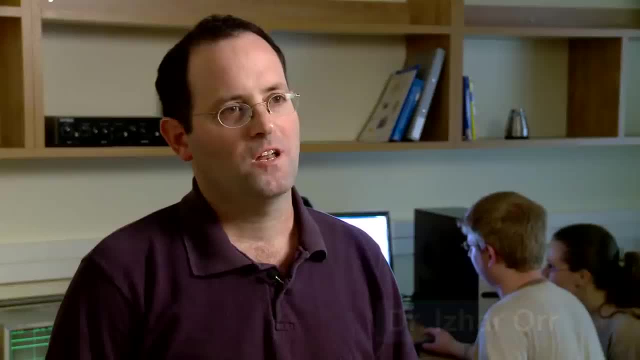 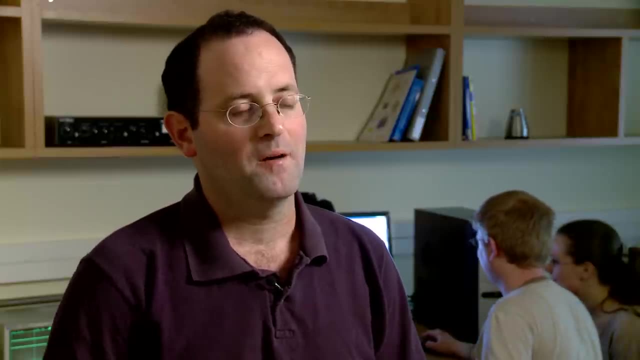 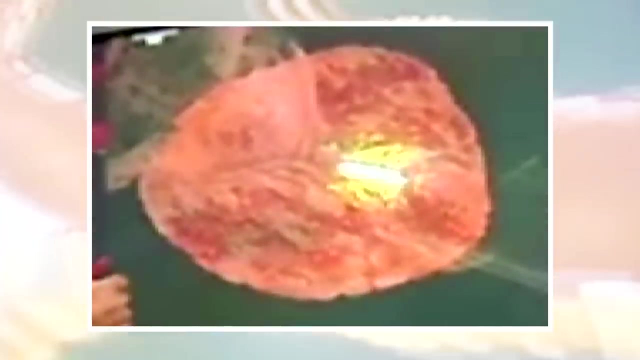 in nature, such as bacteria and sperm cells. Our goal is to develop miniature, micro-scaled robotic swimmers that can be incorporated into mobile human systems such as the circulatory system, the spinal column and the digestive system. These swimmers are designed to perform biomedical tasks such as time-release medication administration. 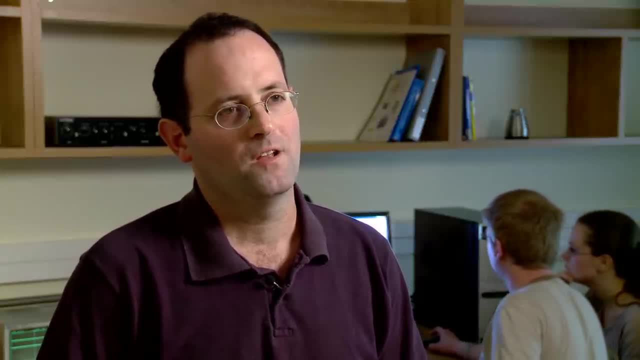 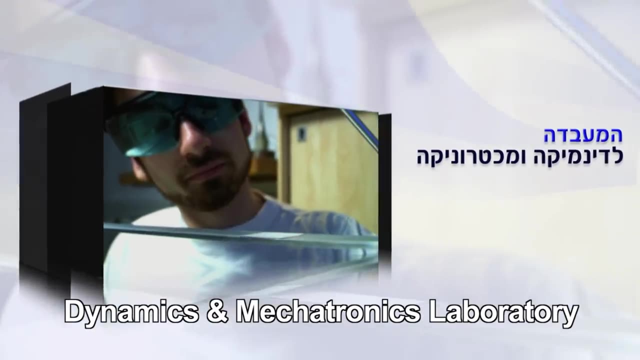 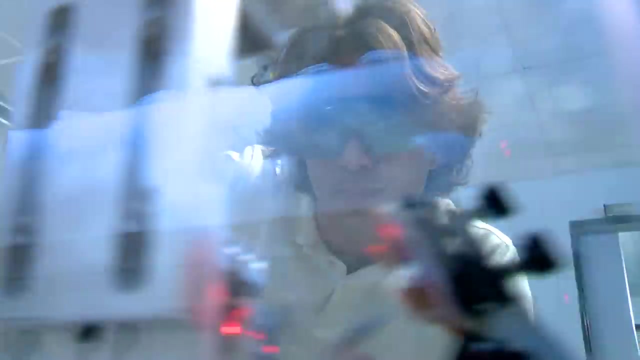 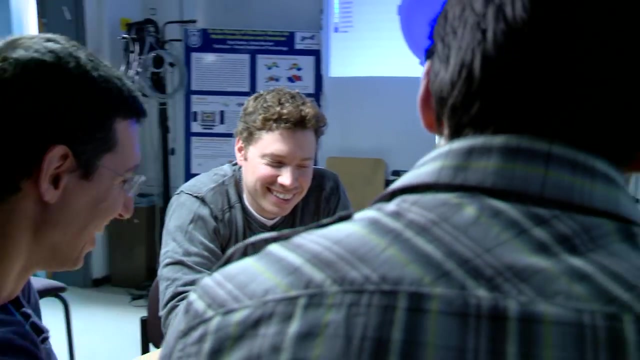 transferring camera images, scanning infected areas and tumors, and even performing localized treatments. The device behind me is an enlarged prototype of a technology that will enable us to create energy from slow movement. Researchers in Professor Yitzhar Bucher's dynamics lab are making waves within solids. 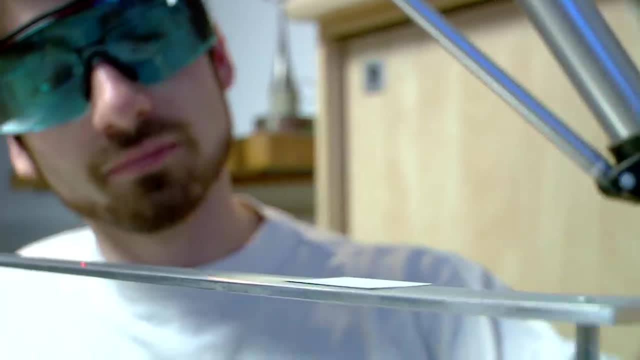 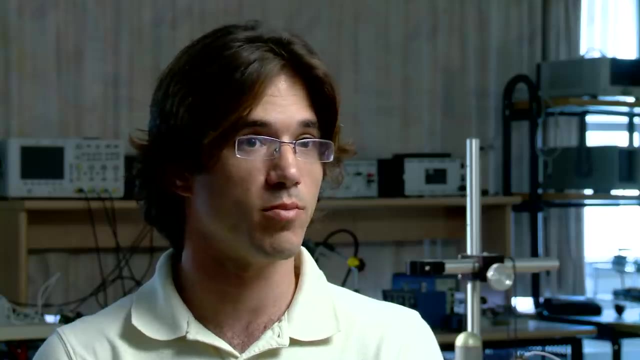 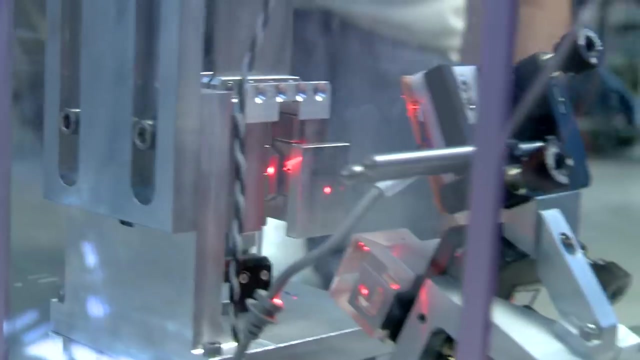 and in the air in order to produce electricity efficiently and transport tiny components and micron-scale swimmers automatically, without the touch of human hands. These movements can be hand, foot or chest movements, or even movements inside the human body, such as the expansion and contraction of the lungs and the beating of the heart. 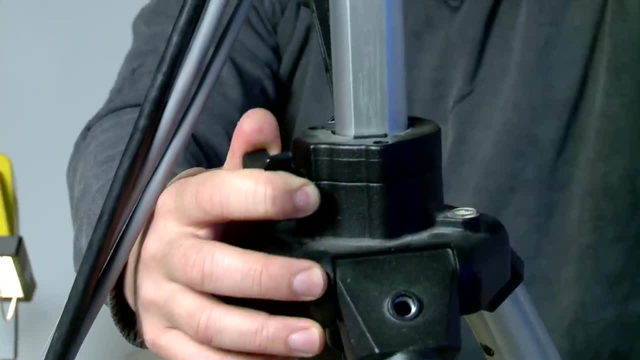 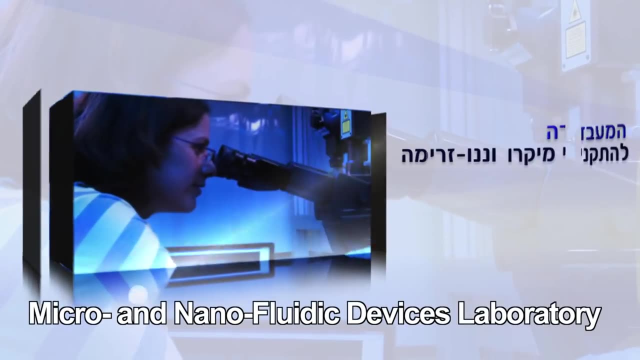 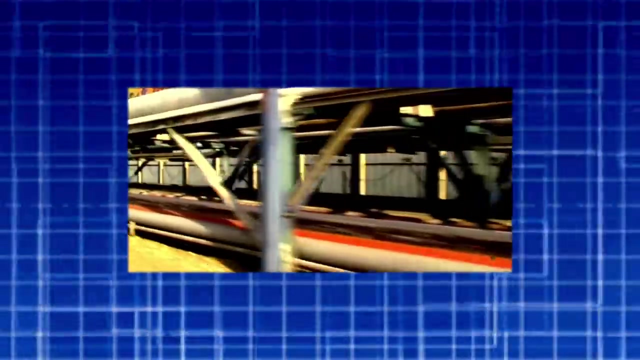 In the future, envelopes will be available to the public. These waves will be capable of moving companies of nanorobots through the human body to target and treat infected areas and ulcers. Imagine a world in which structures such as this one are compressed into a tiny chip measuring. 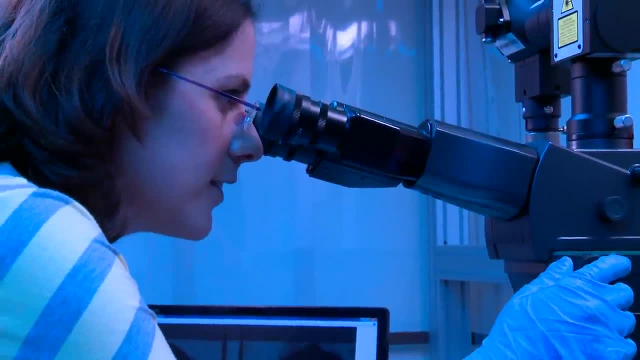 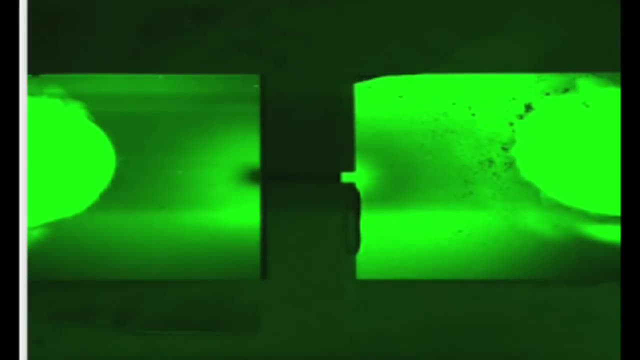 one square centimeter. Researchers in Dr Gilad Yosefone's Micro and Nano-Fluidic Devices Laboratory are investigating ways to manufacture and control the movement of nanorobots. The purpose is actually to take an entire lab and reduce it in size to a miniature scale. 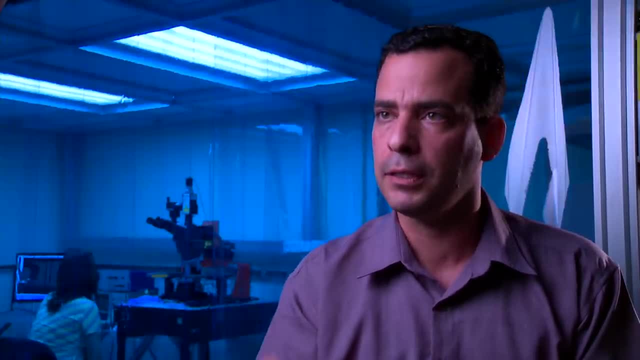 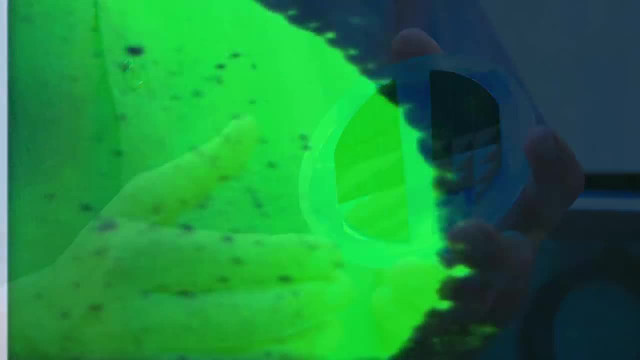 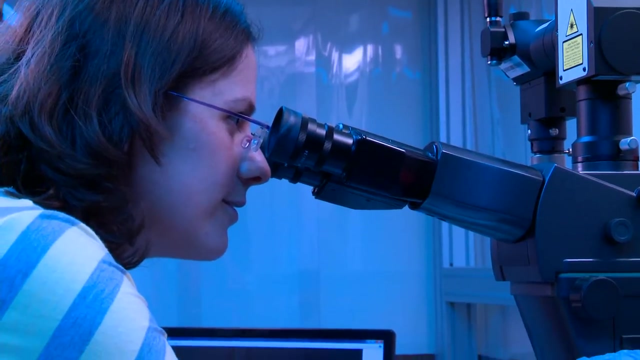 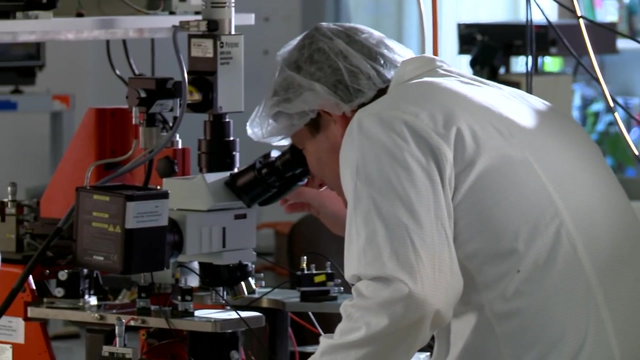 and then to be able to make new discoveries about small amounts of fluid, such as a drop of water or a drop of blood. These miniature devices are characterized by micro and nano channels that can precisely filter nanoparticles and biological molecules. The Microsystems Lab is working on developing micro-mechanic devices for special needs, as 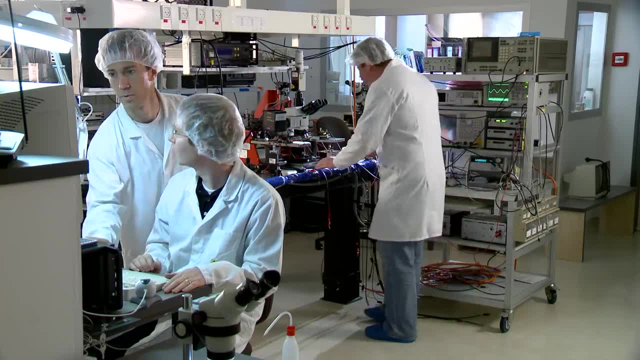 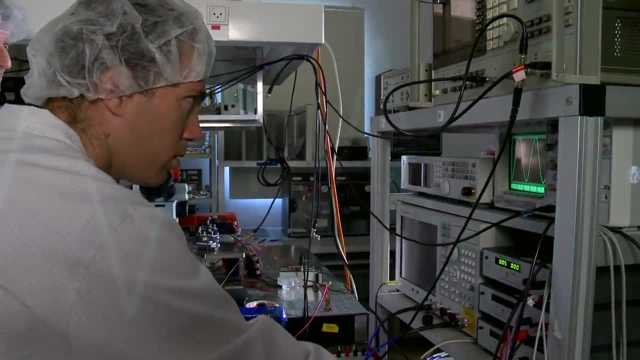 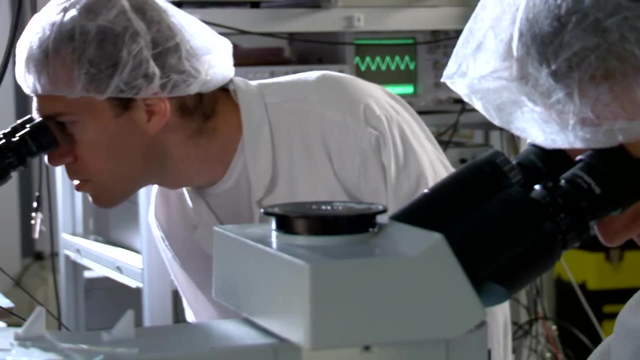 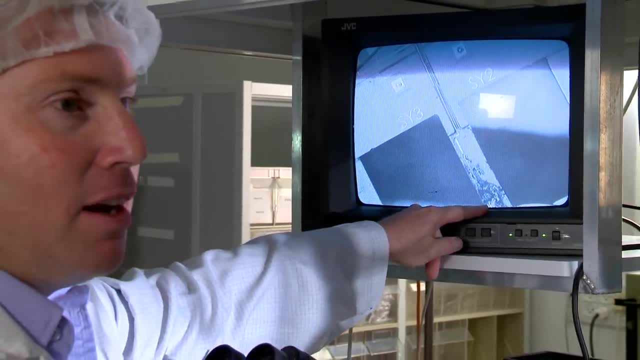 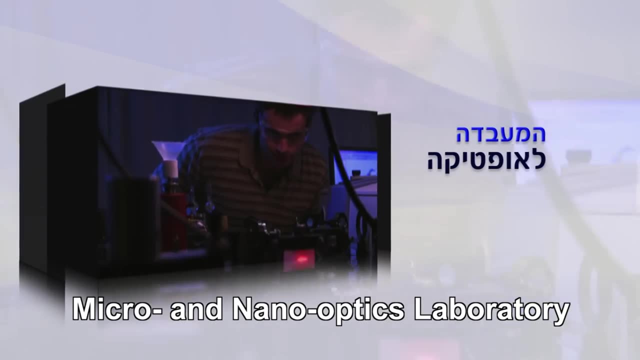 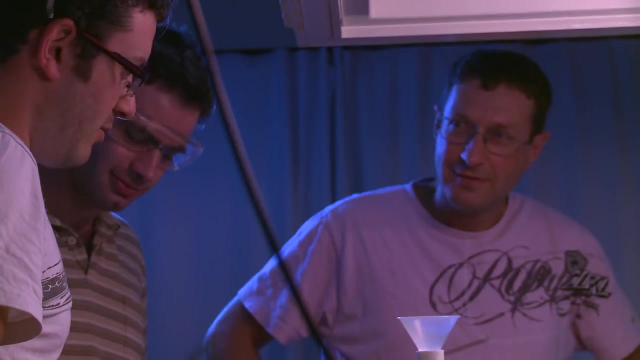 I have been working in the field of micro-mechanics for a long time. I am the CEO of a startup company. The chip we manufacture serves as the core of a miniature projector for cellular phones. In Professor Erez Hasman's Optical Engineering lab, researchers are developing miniature. 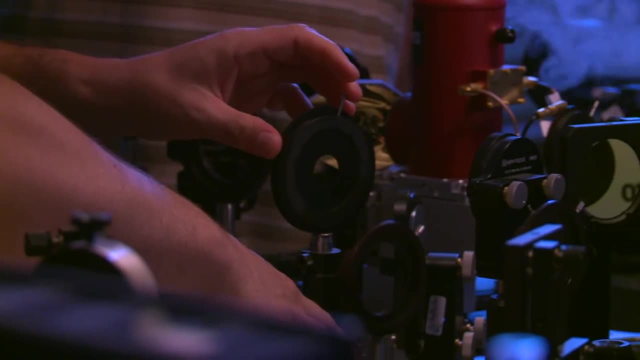 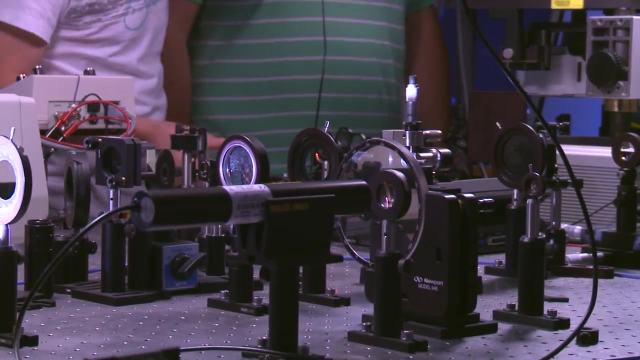 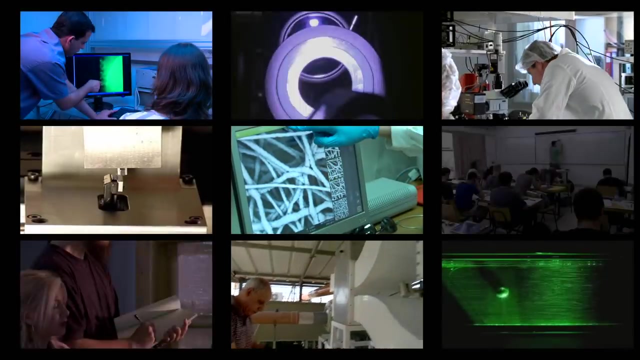 optic components and laser optic mechanic systems for the high-tech industry. The revolutionary technology at Erez is the decision-maker. Technology developed in the Faculty of Mechanical Engineering serves as the basis for building unique opto-nanometric chips. As a result of this extensive research activity, the Faculty has developed many close and productive 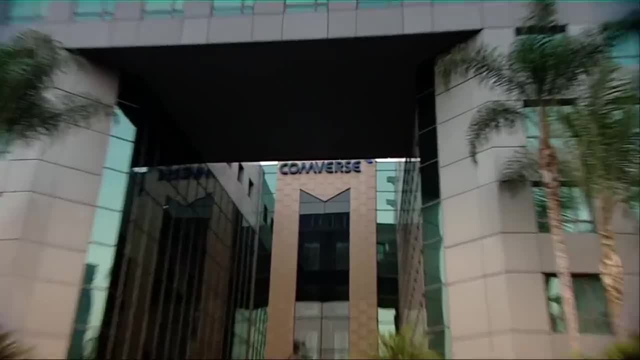 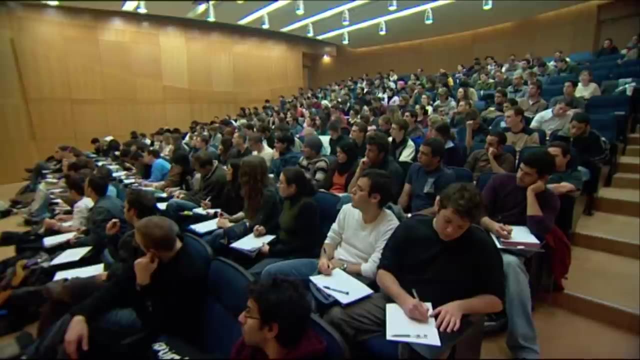 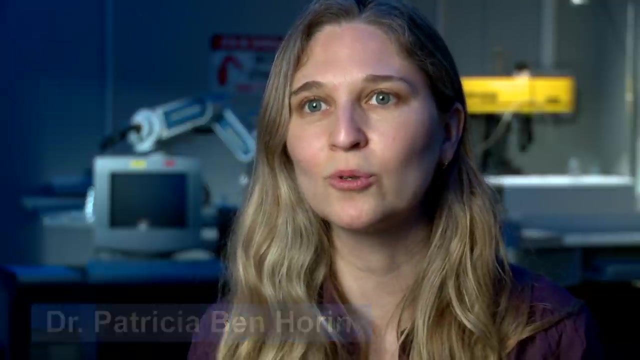 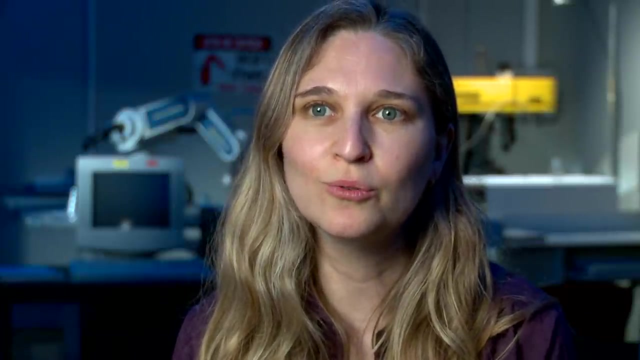 industrial relationships with leading companies in Israel and worldwide. These collaborative relationships facilitate the exchange of research and development knowledge and lay the groundwork for students' future employment. The Faculty of Mechanical Engineering provides excellent tools for setting out on a career as a mechanical engineer. As a systems engineer, I am responsible for seeing the overall picture of an entire project. 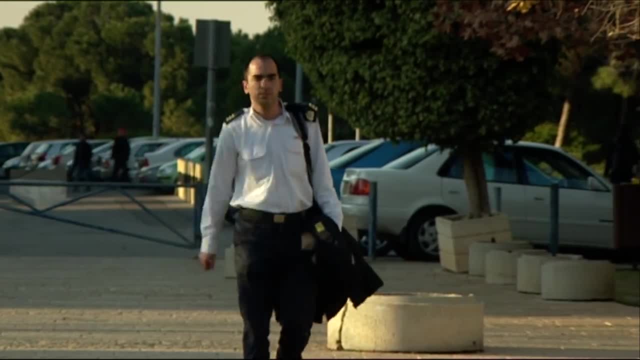 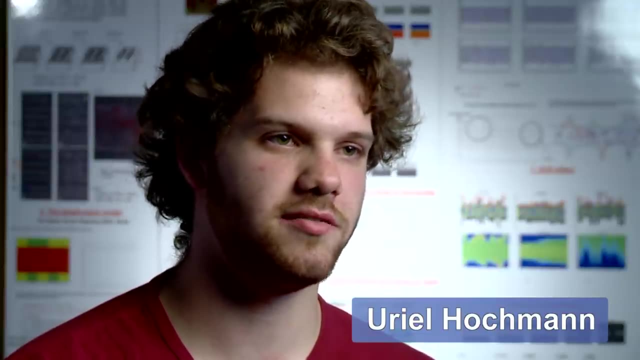 Through the Faculty of Mechanical Engineering's BRAKIM program, the IDF trains its future leaders in research and development. The BRAKIM program is part of the IDF academic reserve and after you complete it you can be posted in any IDF unit. 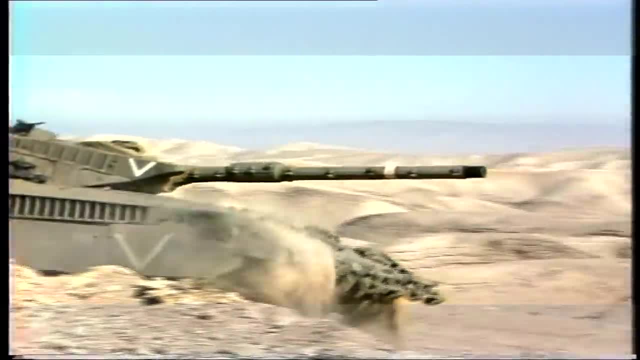 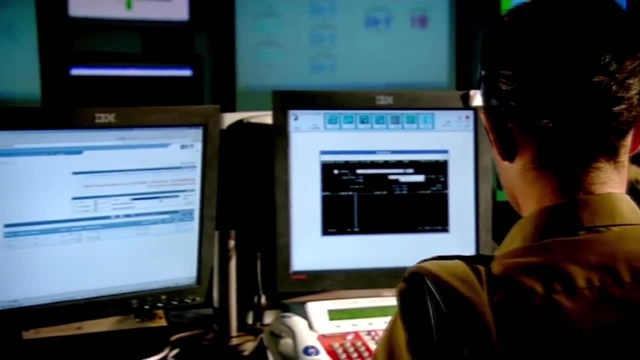 I, for instance, was posted to the Ordnance Corps where the Merkava tanks are developed. The program provided me a great deal of exposure to military and civilian industries. I studied in the IDF academic reserve program and then joined the Intelligence Corps' technology 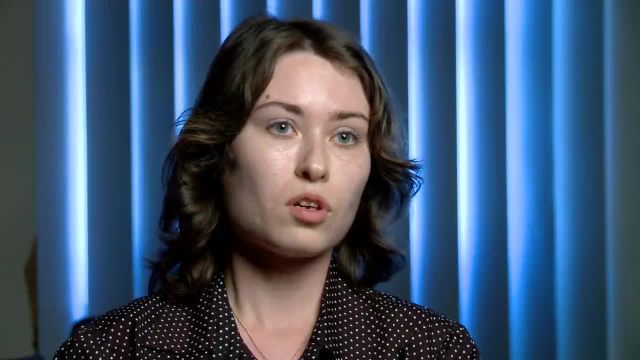 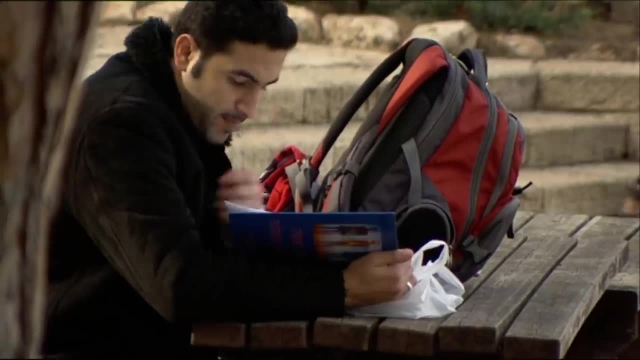 unit At the Technion, I obtained a broad knowledge base in many fields of engineering and then adapted this knowledge for my specific needs at work. Students in the BRAKIM program complete their BA and MA degrees within four years, and 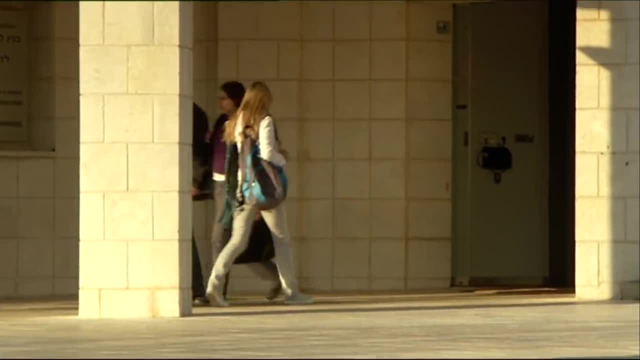 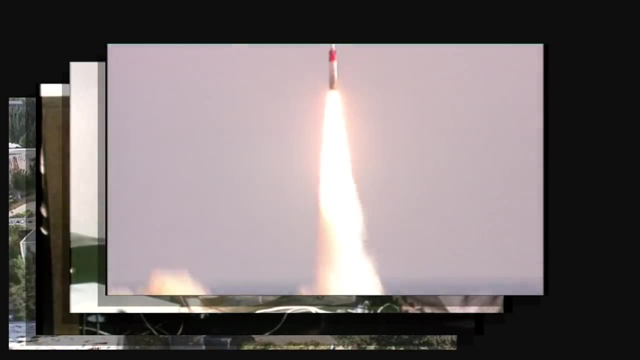 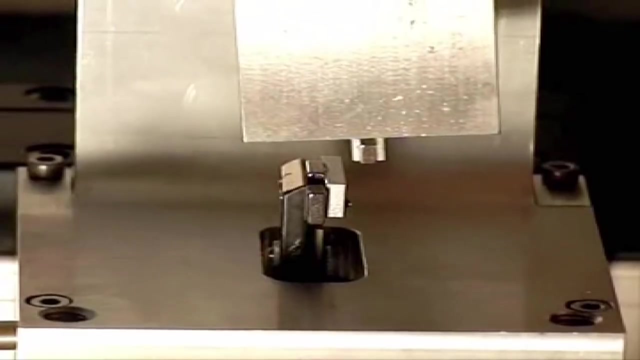 then join the Armed Forces. Since the Faculty of Mechanical Engineering at the Technion was founded in 1935, its more than 8,000 graduates have been major players in Israeli industry, constituting 60% of the country's engineering workforce. 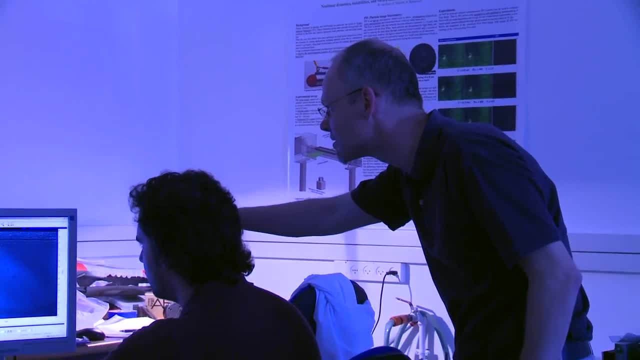 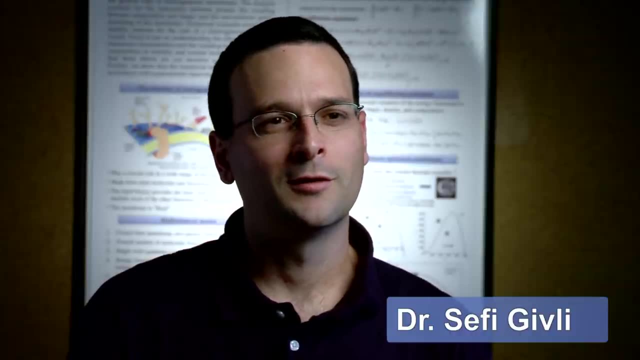 The Faculty constantly strives to keep up with new technological developments and to add innovative fields to its curriculum. The Faculty of Mechanical Engineering has always been my home. I grew up here. I completed my BA, MA and doctorate here. 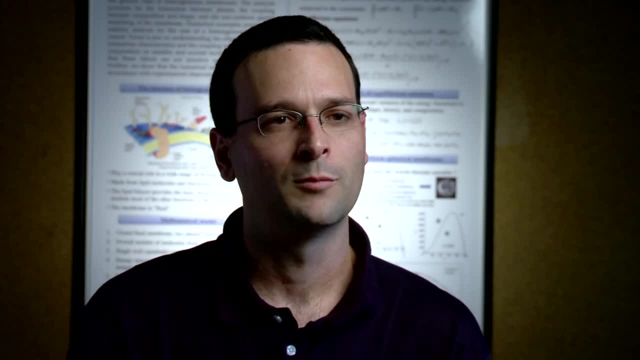 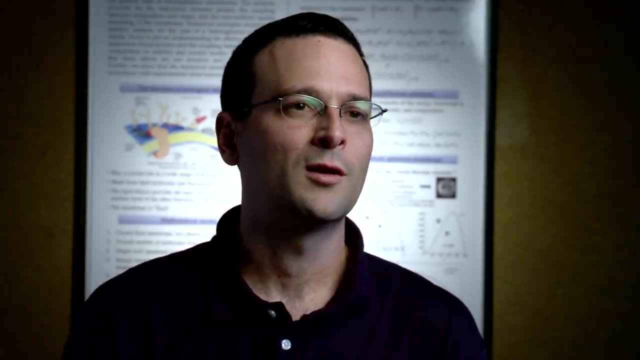 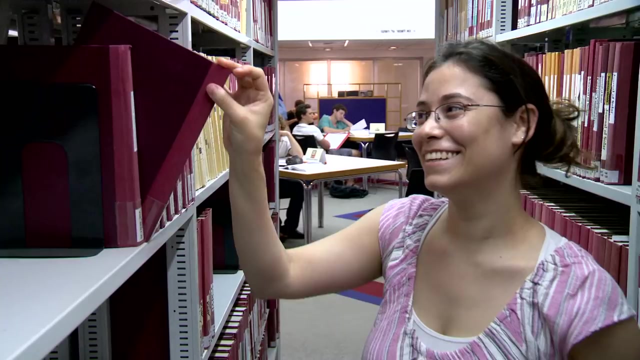 I decided to follow the academic route and did my post-doctorate in the US. The Faculty of Mechanical Engineering at the Technion is a leader in its field in Israel in terms of the quality of its graduates and its researchers. Therefore, it was clear to me that I would want to return.